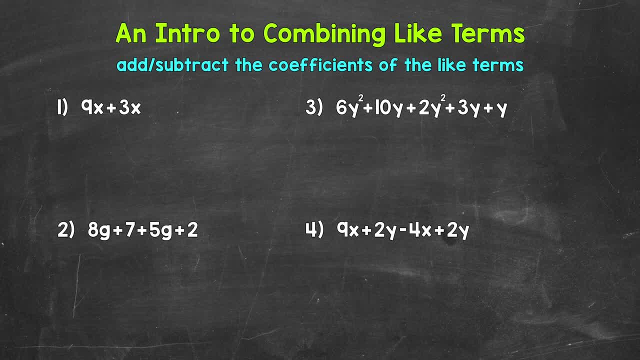 We will start with this basic expression and work our way up. So we have two terms in this expression: 9x and 3x. Both terms have the same variable of x and these variables of x are to the same power. Remember, when we don't have an exponent attached to a variable. 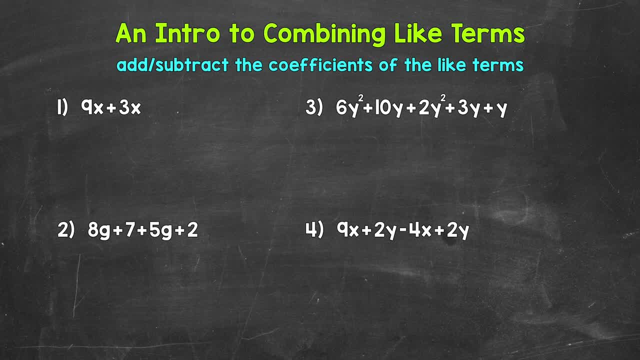 there is an understood exponent of 1.. Anything to the power of 1 is just itself. So 9x and 3x are like terms. Now, when we combine like terms, all we need to do is add or subtract the coefficients. 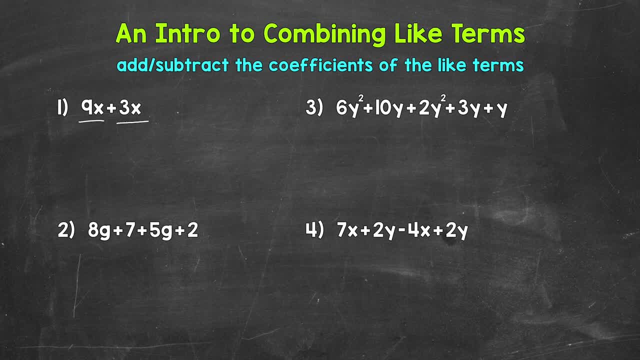 the numbers in front of the variables. The coefficients in number one are 9 and 3.. We have a positive 9x, We have a positive 3x, So let's add those coefficients. 9 plus 3 is 12.. 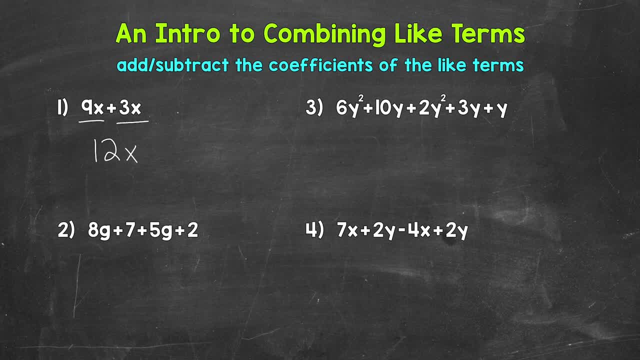 And then we have the variable of x, And that's it. We took those two like terms, 9x and 3x, and combined them into one term: 12x. 12x is equivalent to 9x plus 3x. 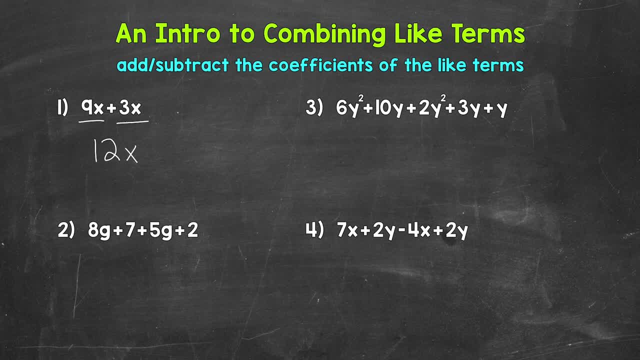 So we didn't change the value of the expression. So 12x is our final simplified expression. Let's move on. Let's move on to number two, where we have 8x plus 7x plus 5x plus 2x. 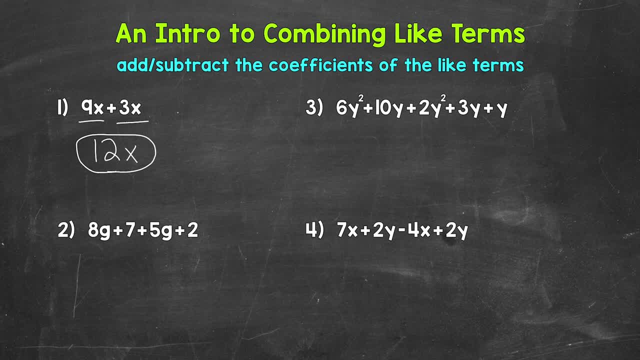 Are there any like terms that we can combine in order to simplify this expression? Yes, we have 8x and 5x. Both of those terms have that variable of x, And then we have constant terms 7x and 2x. 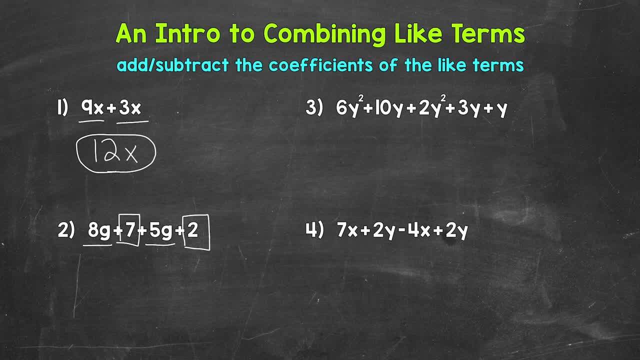 I'll box in the constant terms to separate them from the, The 8x and the 5x. Now we can combine like terms: We have 8x plus 5x, That gives us 13x, And then we have 7x plus 2x. 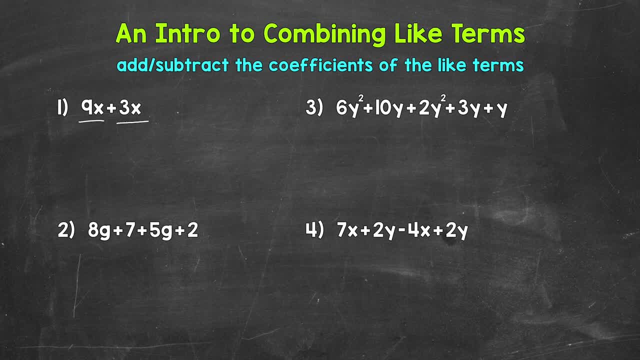 the numbers in front of the variables. The coefficients in number one are 9 and 3. We have a positive 9x Plus a positive 3x, So let's add those coefficients. 9 plus 3 is 12.. 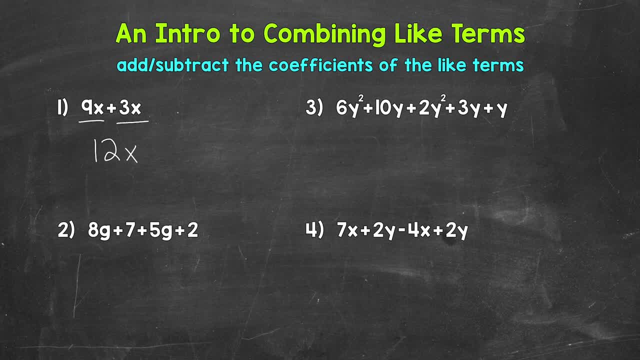 And then we have the variable of x, And that's it. We took those two like terms, 9x and 3x, and combined them into one term: 12x. 12x is equivalent to 9x plus 3x. 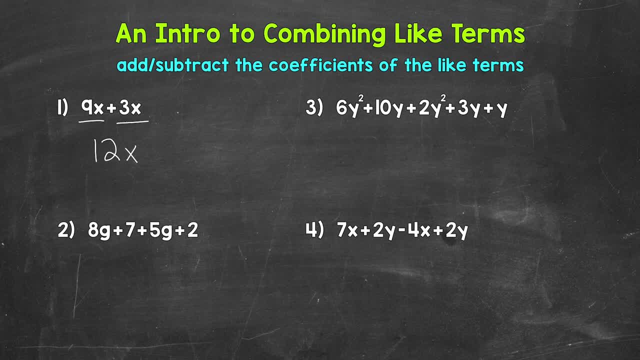 So we didn't change the value of the expression. So 12x is our final simplified expression. Let's move on To number two, where we have 8x plus 7x plus 5x plus 2x. Are there any like terms that we can combine in order to simplify this expression? 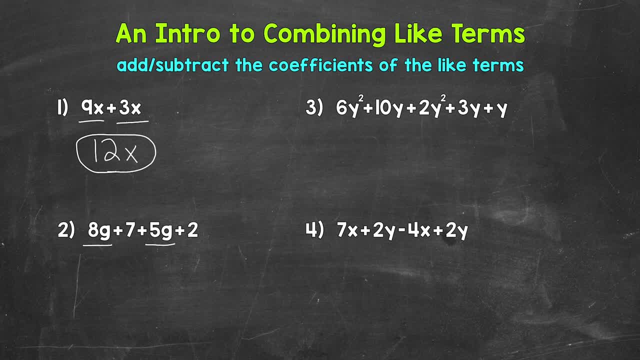 Yes, we have 8x and 5x. Both of those terms have that variable of x. And then we have constant terms: 7x and 2x. I'll box in the constant terms to separate them From the 8x and the 5x. 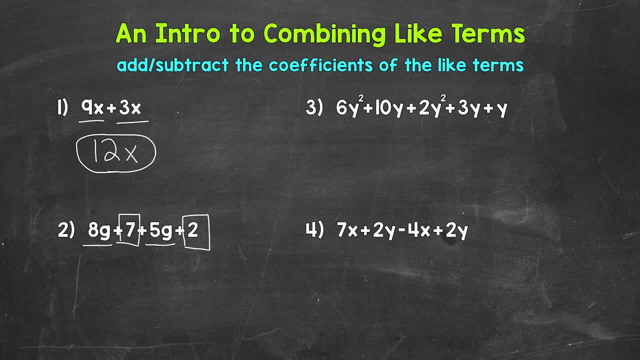 Now we can combine like terms: We have 8x plus 5x, That gives us 13x. And then we have 7x plus 2x, That gives us 9x. So we end up with 13x plus 9x. 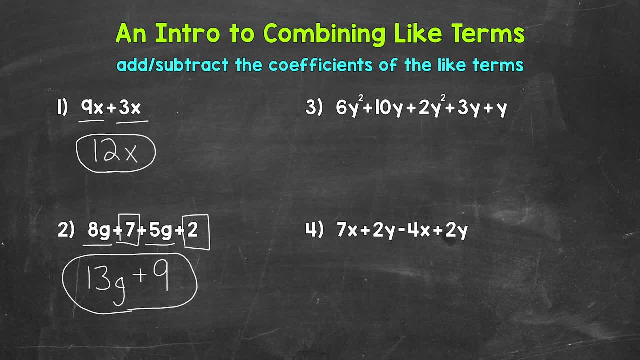 And that's our simplified expression. That expression of 13x plus 9x is equivalent to the original expression. We were just able to simplify The original expression by combining like terms. We started with four total terms, But we were able to combine like terms. 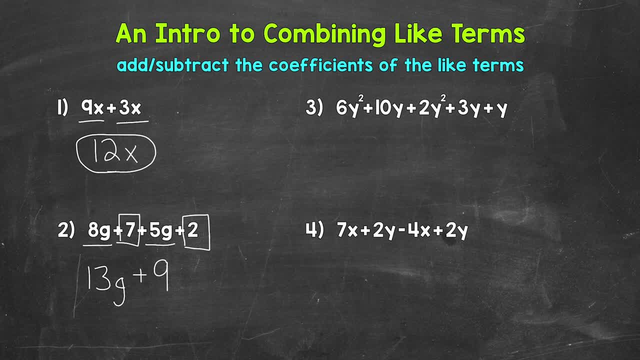 That gives us 9x. So we end up with 13x plus 9x, And that's our simplified expression. That expression of 13x plus 9x is equivalent to the original expression. We were just able to simplify the. 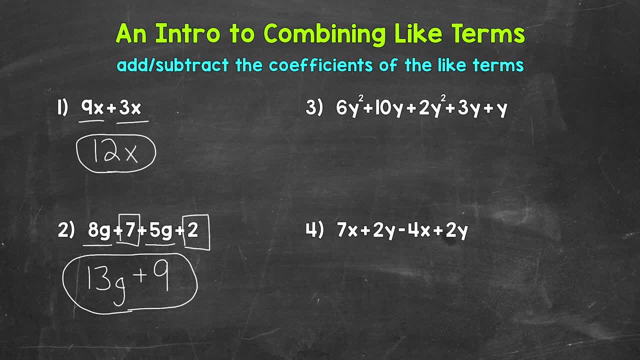 The original expression by combining like terms. We started with four total terms, but we were able to combine like terms And now we only have two total terms. Let's move on to number three, where we have 6y squared plus 10y plus 2y squared plus 3y plus y. 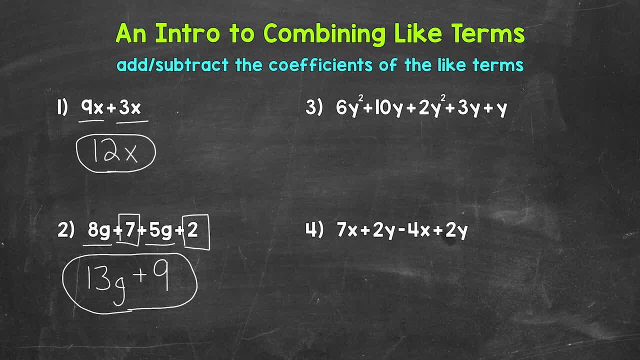 Let's find any like terms that we can combine. We'll start with 6y squared. 2y squared is a like term. Both of those terms have that variable of y to the power of 2.. Now do we have any other like terms within this algebraic expression that we can combine? 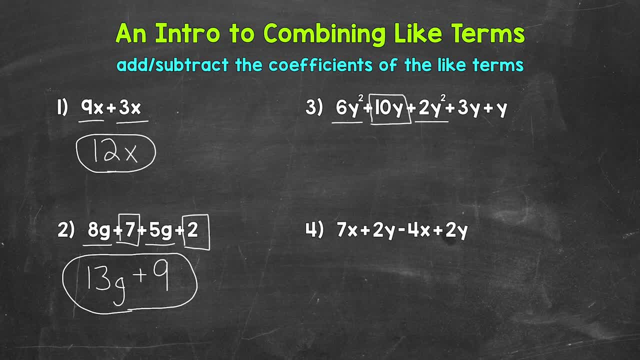 Yes, 10y, And I will box these terms in in order to separate them from the y squared terms: 3y And then y. Now I do want to mention this term right here. the y, the variable by itself. 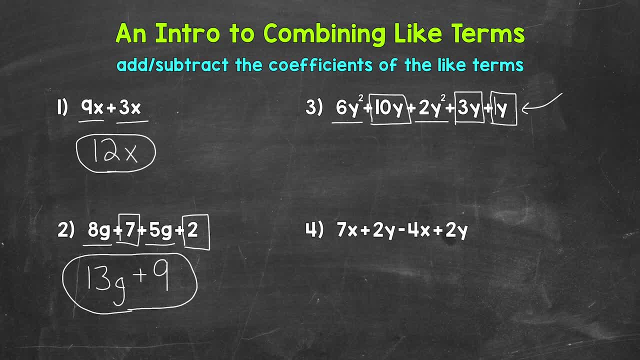 The coefficient is 1.. We don't have a coefficient written in front Whenever you see that the coefficient is 1.. There is an understood 1 in front of a variable And it can be helpful to write that 1 in there when you combine like terms. 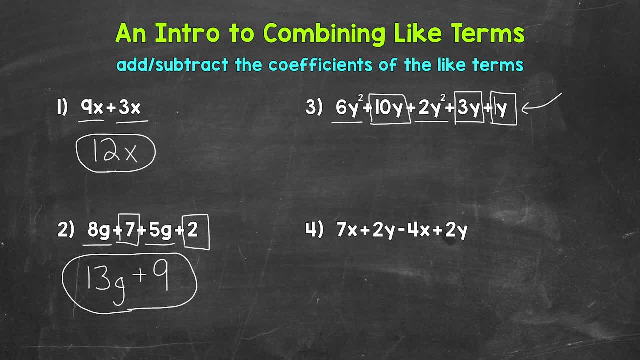 So you can always write that 1 if you would like. Now, since this algebraic expression has five terms and we are working our way up to more complicated algebraic expressions, we're going to use a strategy to help us organize the expression before we combine like terms. 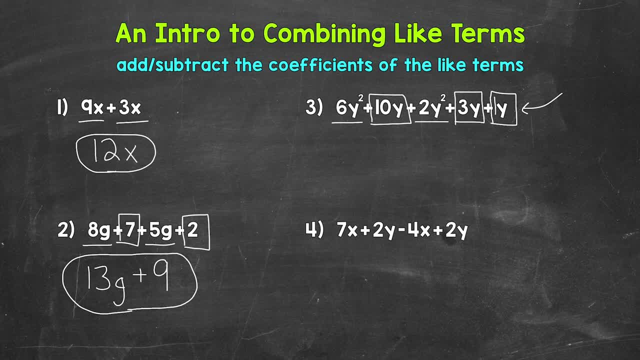 We are going to rearrange and rewrite the expression and put the like terms next to each other. I'll start with 6y squared plus the like term of 2y squared plus. now we have the y terms, so 10y plus 3y. 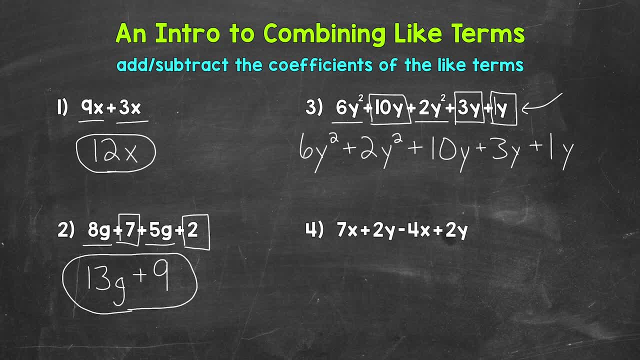 So now all of the like terms are next to each other and it's a little easier to see what we can combine. So this is a strategy to keep in mind. Now, do you have to do this step in order to combine like terms? 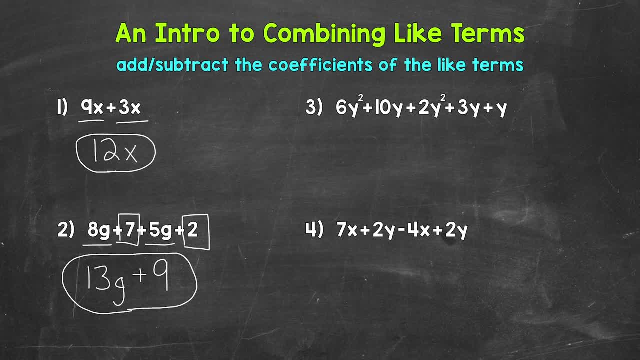 And now we only have two total terms. Let's move on to number three, where we have 6y squared plus 10y plus 2y squared plus 3y plus y. Let's find any like terms that we can combine. 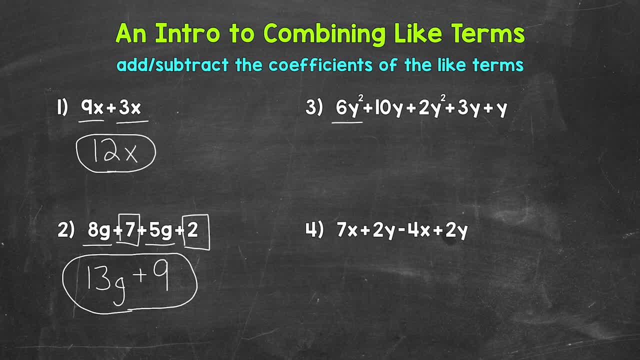 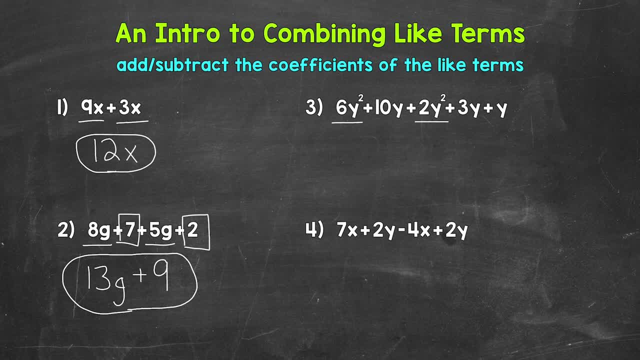 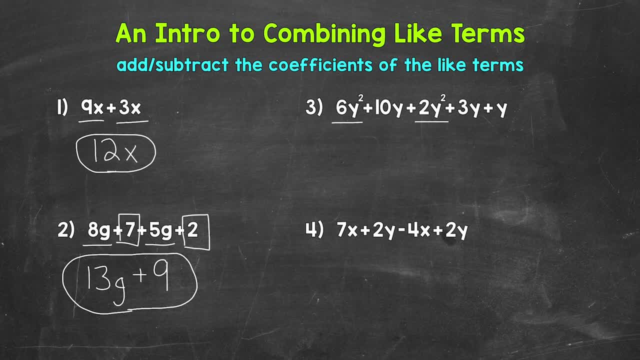 Now, do we have any other like terms within this algebraic expression that we can combine? Yes, 10y, And I will box these terms in in order to separate them from the y squared terms 3y And then y. 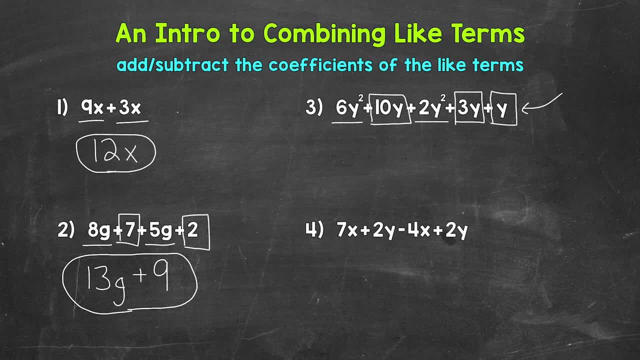 Now I do want to mention this term right here: the y, the variable by itself, the coethype Coefficient is 1.. We don't have a coefficient written in front Whenever you see that the coefficient is 1.. 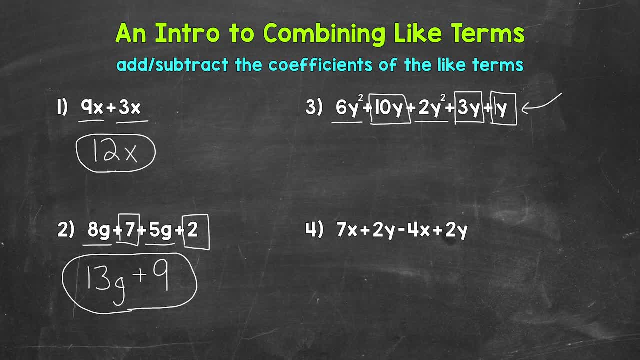 There is an understood 1 in front of a variable And it can be helpful to write that 1 in there when you combine like terms. So you can always write that 1 if you would like Now, since this algebraic expression has 5 terms and we are working our way up to more. 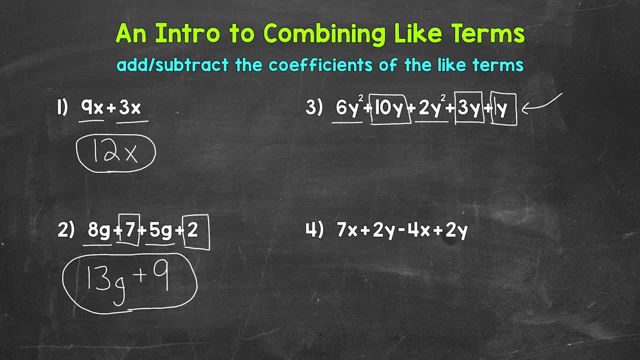 complicated terms. We are going to use a strategy to help us organize the expression. before we combine like terms, We are going to rearrange and rewrite the expression and put the like terms next to each other. I'll start with 6y squared plus the like term of 2y squared plus. now we have the y. 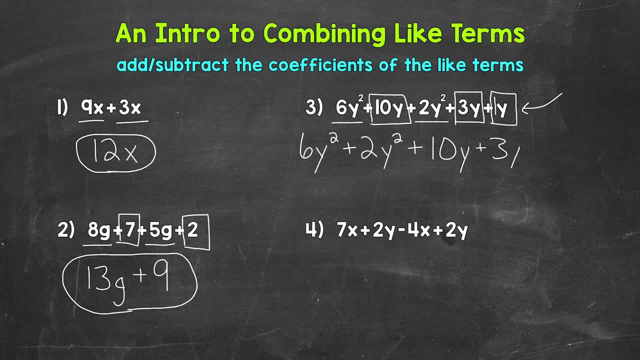 terms, so 10y plus 2y, 3y plus 1y. so now all of the like terms are next to each other and it's a little easier to see what we can combine. So this is a strategy to keep in mind. 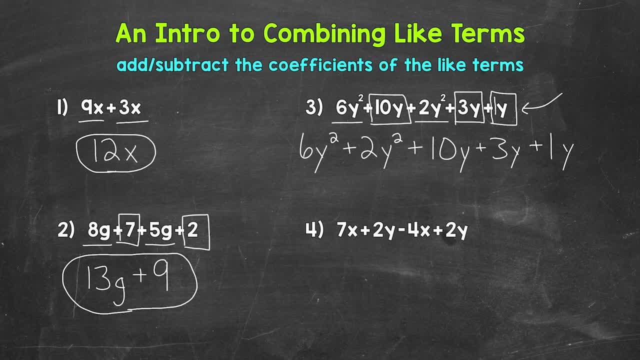 Now, do you have to do this step in order to combine like terms? No, but it can be helpful. Now we can combine like terms. We will start with 6y squared plus 2y squared, So add the coefficients: 6 plus 2 is 8, and then we have y squared plus. now we can combine the y terms. 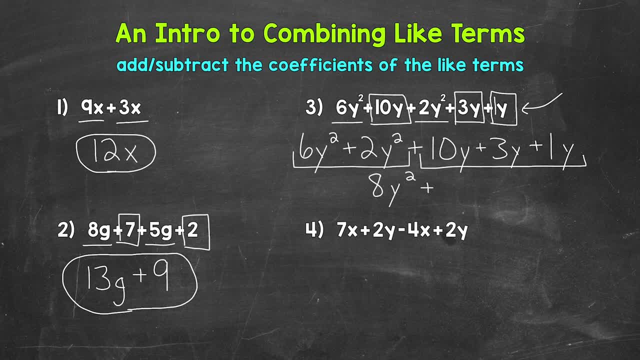 So we have 10 plus 3 plus 1, 10 plus 3 is 13, plus 1 is 14.. So we get 8y squared plus 14y, and that's the simplified expression. We now have an equation. 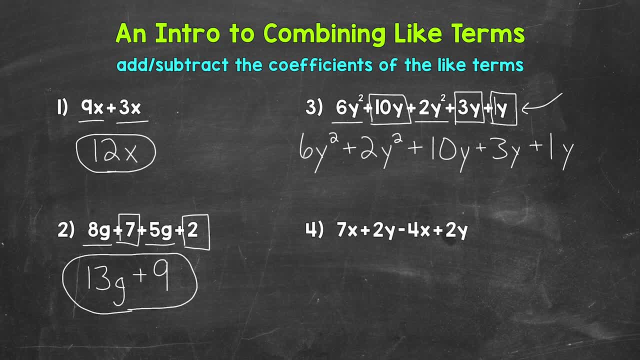 No, but it can be helpful. Now we can combine like terms. We will start with 6y squared plus 2y squared, so add the coefficients: 6 plus 2y squared 2 is 8, and then we have y squared plus. now we can combine the y terms. 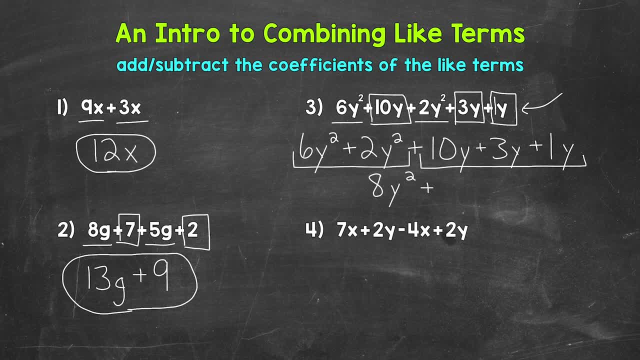 So we have 10 plus 3 plus 1.. 10 plus 3 is 13, plus 1 is 14.. So we get 8y squared plus 14y and that's the simplified expression. We now have an equivalent expression that is simplified. 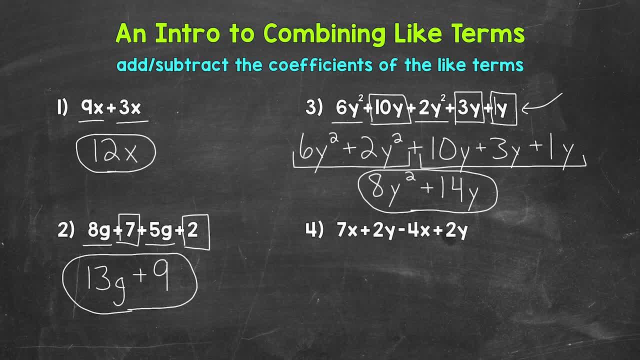 It's simpler than the original. We simplified the expression. We went from 5 terms to 2 terms. Let's move on to number 4, where we have 7x plus 2y minus 4x plus 2y. 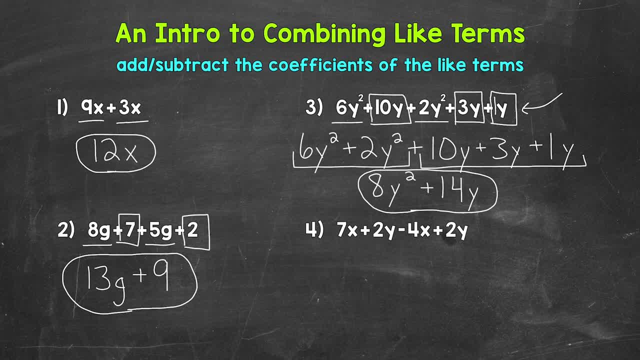 Let's find any like terms that we can combine. We will start with 7x and negative 4x. Now, when we combine like terms, a term is going to take the sign that's in front of it. So this is negative 4x. 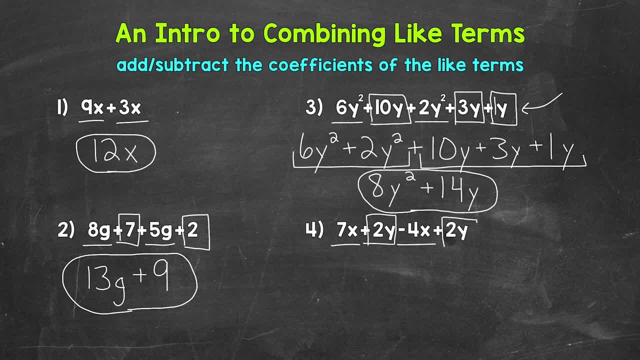 Then we have 2y and 2y, So let's box those terms in in order to separate them from the x terms. Now we can rewrite this expression with the like terms next to each other. We will start with 7x minus 4x. 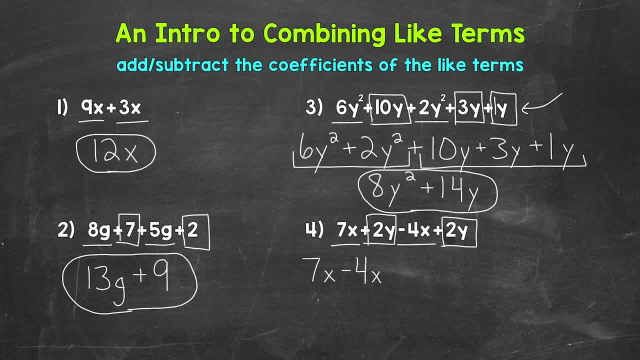 So we have a negative 4x there. Make sure to bring the sign that's in front of the term with it When we rewrite the expression plus 2y. so now we have the y terms plus another 2y. 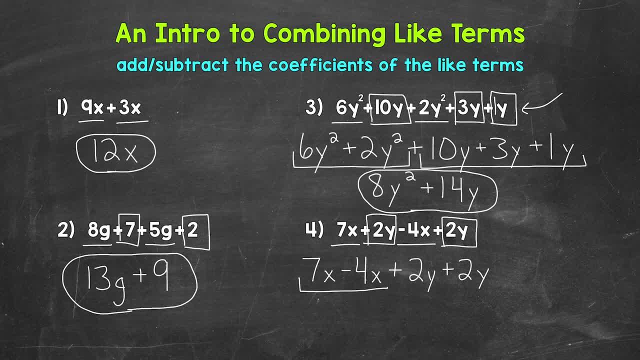 Now we can combine like terms, So we have 7x minus 4x, Or you can think of this as 7x being combined with negative 4x. however you want to think about it, 7 minus 4 is 3.. 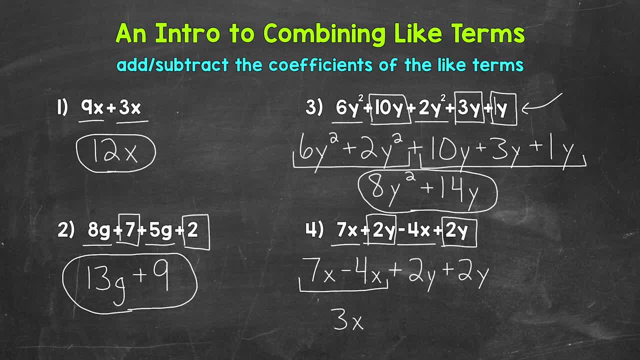 And then we have the x, Or if you're thinking about it as 7x combined with a negative 4x, 7 and negative 4 give us 3 as well. Then we have our 2y plus 2y. 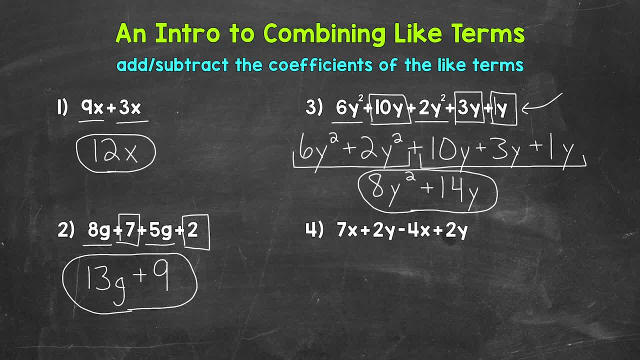 We now have an equivalent expression that is simpler than the original. We simplified the expression. We went from 5 terms to 2 terms. Let's move on to number 4, where we have 7x plus 2y minus 4x plus 2y. 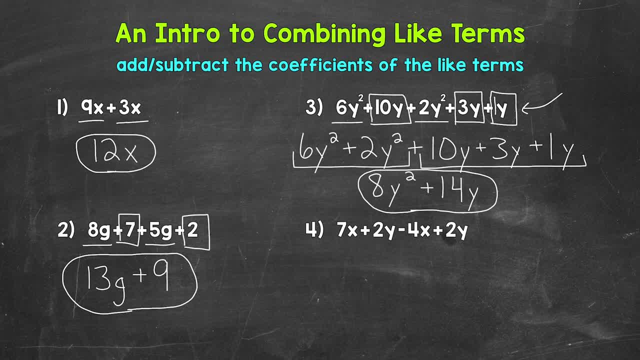 Let's find any like terms that we can combine. We will start with 7x and negative 4x. Now, when we combine like terms, a term is going to take the sign That's in front of it. So this is negative 4x. 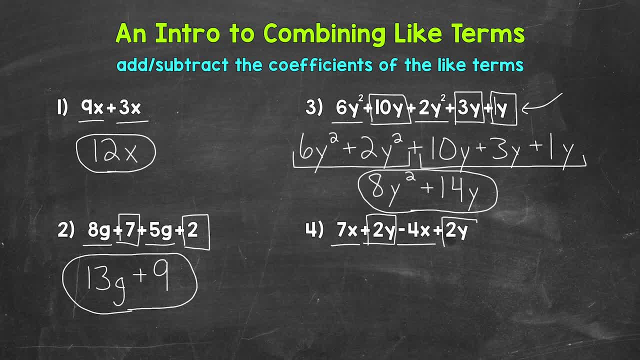 Then we have 2y and 2y, So let's box those terms in in order to separate them from the x terms. Now we can rewrite this expression with the like terms next to each other. We will start with 7x minus 4x. 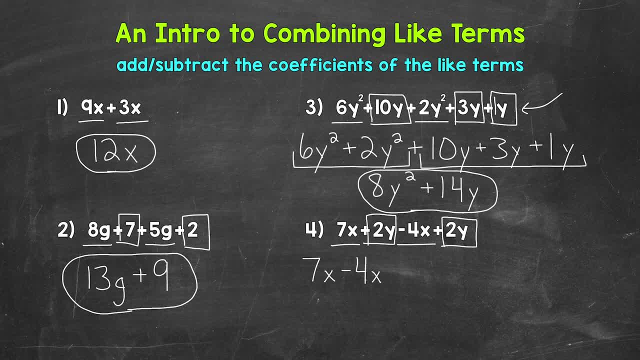 So we have a negative 4x there. Make sure to bring the sign That's in front of the term with it When we rewrite the expression plus 2y. So now we have the y terms plus another 2y. Now we can combine like terms. 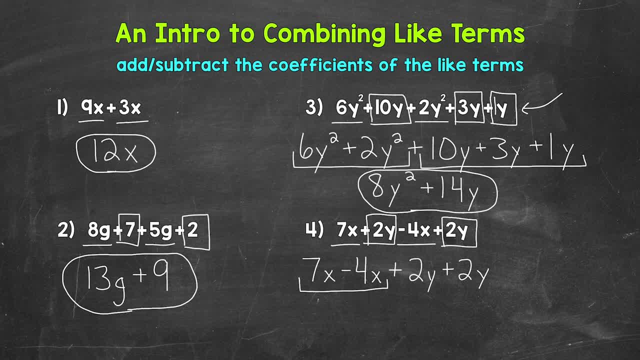 So we have 7x minus 4x, or you can think of this as 7x being combined with negative 4x. However you want to think about it, 7 minus 4 is 3.. And then we have the x. 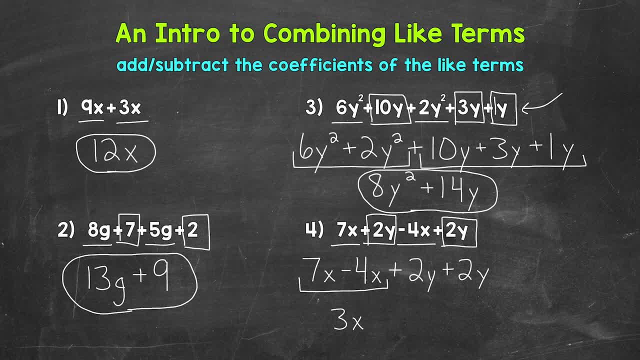 Or if you're thinking about it as 7x combined with a negative 4x, 7 and negative 4 give us 3 as well. Then we have our 2y plus 2y. That gives us plus 4y. 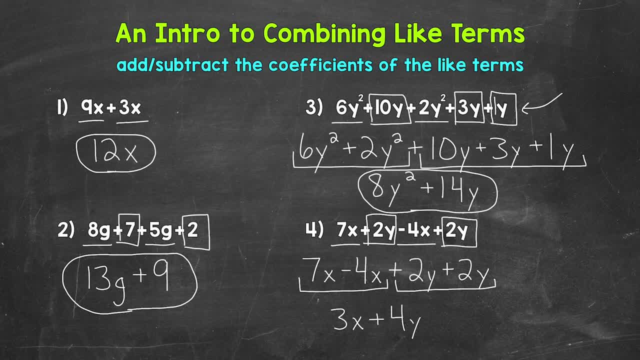 That gives us plus 4y, So we end up with 3x plus 4y, And that's our simplified expression. We went from 4 total terms to 2 total terms by combining like terms, So we end up with 3x plus 4y. 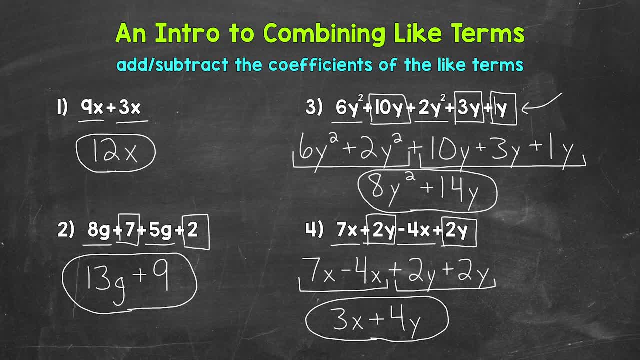 And that's our simplified expression. We went from 4 total terms to 2 total terms by combining like terms. 3x plus 4y is equivalent to the original expression. We were just able to again simplify this expression by combining like terms: 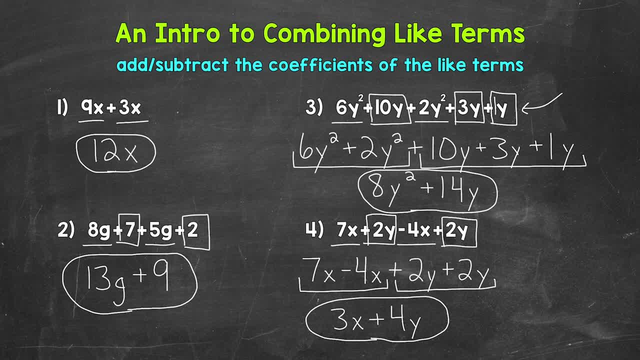 Now I also want to go through simplifying this expression, a slightly different way to start off, And that's by rewriting the original expression with only addition, separating the terms. We do this by changing any subtraction to adding the opposite. The benefit of having all terms separated or subtracted is that we can do this by adding. 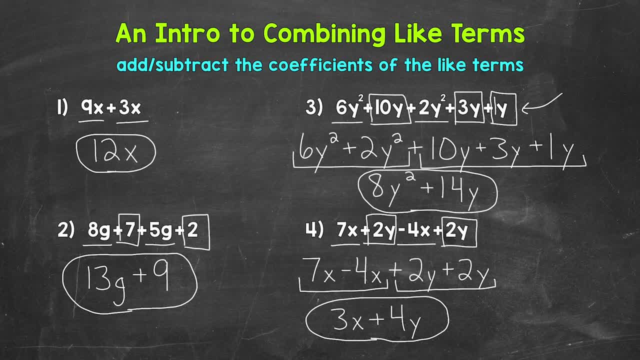 the opposite. Just regarding individuals being separated only by addition, is that it's a little simpler to identify all of the terms, especially any negative terms. I kind of organizes the expression and helps any negatives stand out. Alright, I'll rewrite the equation off to the side here. so 7x plus 2y minus 4x plus. 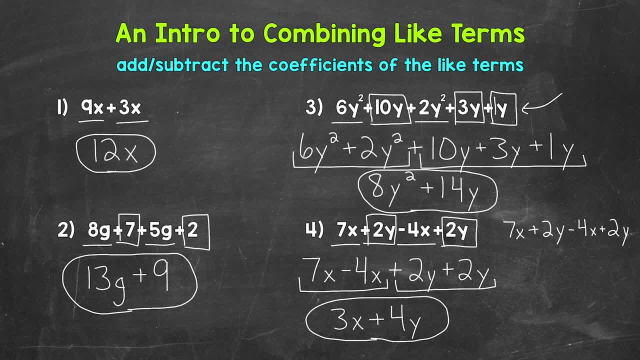 2y y. So let's rewrite subtraction as adding the opposite. So adding the opposite of a positive 4x is a negative 4x, So adding the opposite. Let's rewrite the expression with that change. So we have 7x plus 2y plus negative 4x plus 2y. Let's rewrite that expression with like terms. next. 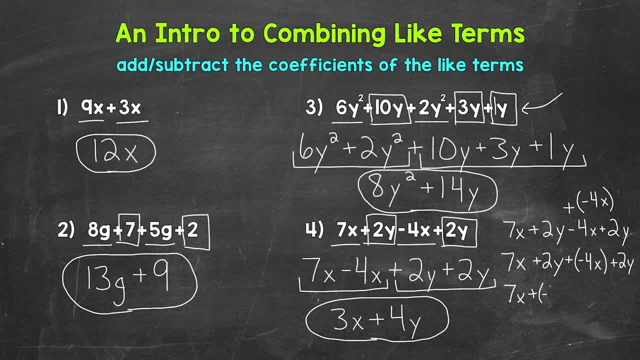 to each other, So 7x plus negative 4x plus 2y plus 2y. Now we can combine like terms: We have 7x plus negative 4x plus 2y, 7x plus negative 4x, That gives us 3x. And then we have 2y plus 2y, So that gives us plus 4y. 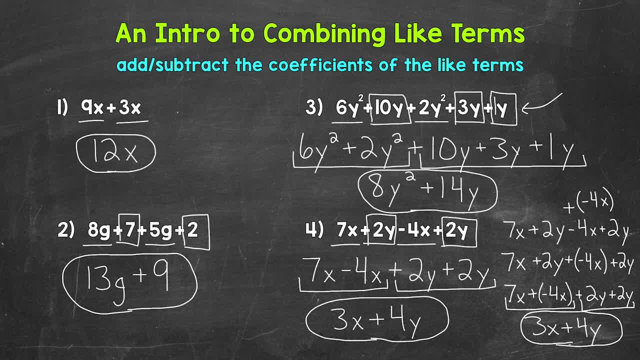 3x plus 4y that way as well. So that's just another strategy to be aware of. So there you have it. There's an introduction to combining like terms. I hope that helped. Thanks so much for watching. Until next time. 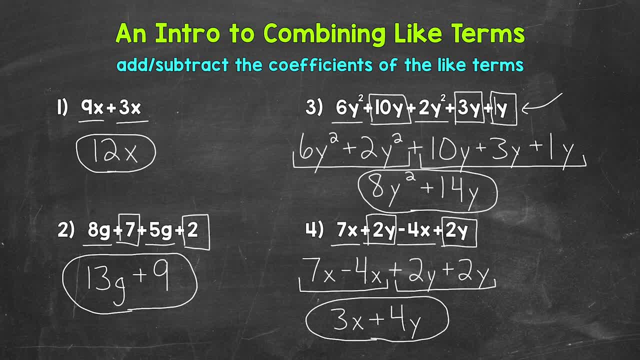 So we end up with 3x plus 4y, And that's our simplified expression. We went from 4 total terms to 2 total terms. So that's our simplified expression. We went from 4 total terms to 2 total terms. 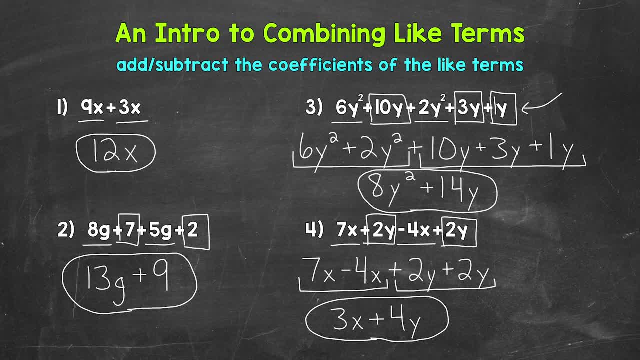 And we're going to go through this again. We were able to simplify this expression by combining like terms: 3x plus 4y is equivalent to the original expression. We were just able to again simplify this expression by combining like terms. Now I also want to go through simplifying this expression a slightly different way to.